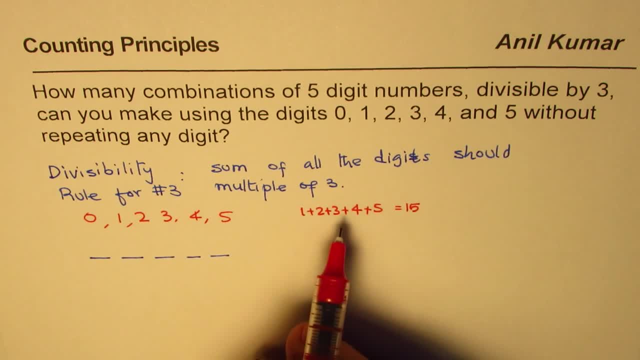 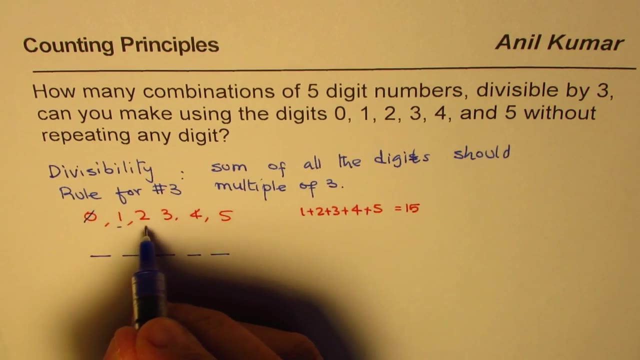 when put together form a number or a divisible, So number. to put together 4 and 7, this will, which is multiple of three. right now, out of six we have to select any five. so let's disregard zero for the first time, and then we will see how to make a number using these five digits. so we'll 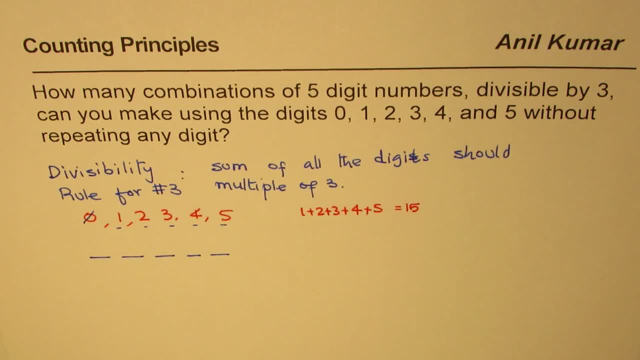 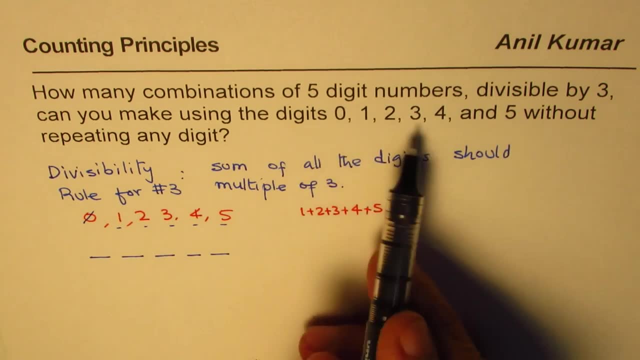 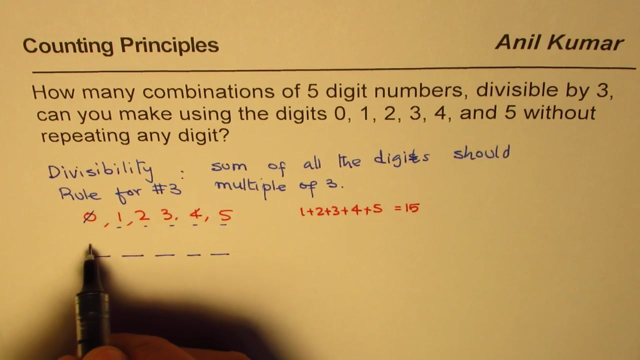 take one, two, three, four and five. now, if i have to form a five digit number using one, two, three, four, five, we have to disregard one right because we are given six digits. then, to fill in the first position, we could fill with either one of these fives. once the number has been filled, we are left. 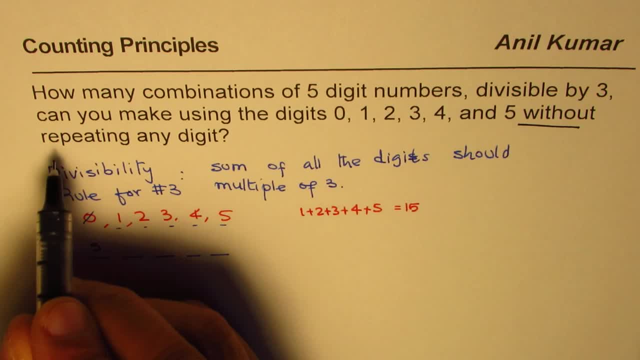 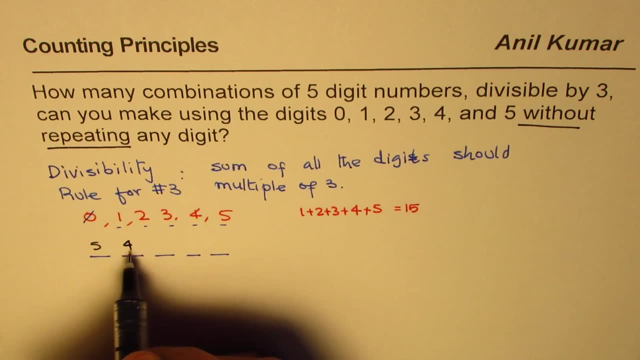 with four without repeating right. remember that without repeating. so we cannot use one number which we have used here. so we are left with four, and once we place two numbers, we are left with three, and then with two, and then with one. that gives us a number that is equal to four, and so 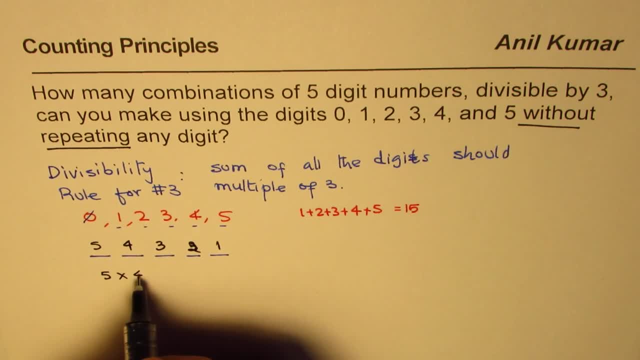 gives total number of combinations as 5 factorial, or 5 times 4 times 3 times 2 times 1, which is 5 times 4, 20, 20 times 3, is 60 times 2 is 120. So we get 120 combinations of these numbers. 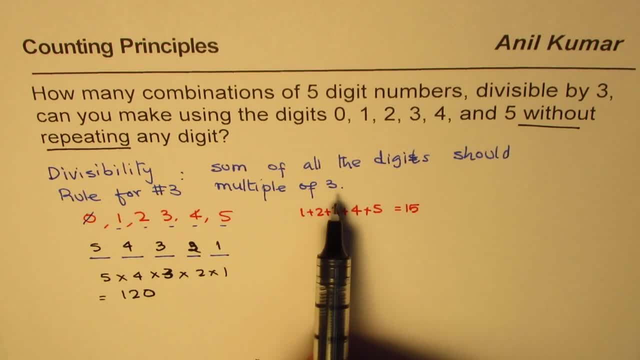 which will all be multiple of 3. right, which will all be multiple of 3.. So that is one way we can use these six numbers. Now let us see: can we use 0, 2, 3, 5 and 4. that is disregard 1.. So if I take 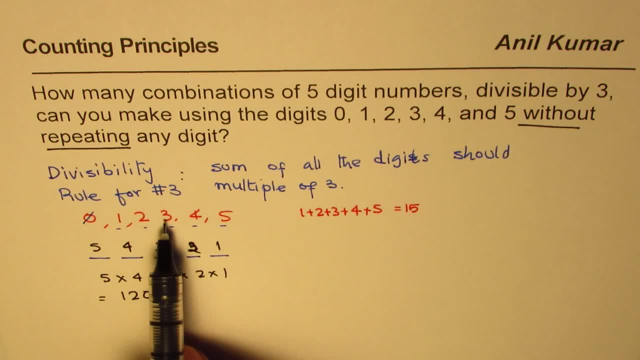 away 1, then the sum of the numbers will be: 2 plus 3 is 5 plus 4. 9 plus 5 is 14, 1 less than 15.. Well, 14 is not the multiple, so we cannot work with that. If we take away 2 from the list, then the 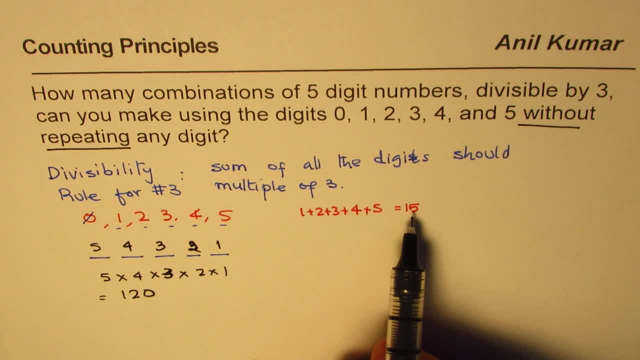 sum will be 13.. If we take away 2 from the list, then the sum will be 13.. If we take away 2 from the list, then the sum will be 13.. If we take away 3, sum will be 12. 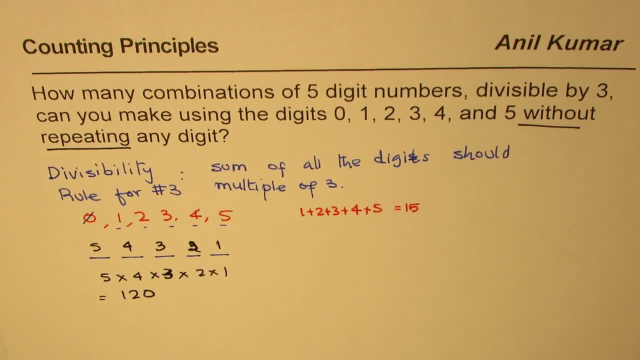 12 is a multiple right, So we could actually form the numbers using 0, 1, 2. taking away 3 leaves us with 4 and 5.. So these five digits, right. So let us see how many numbers can we make with these five. We want to make five digit numbers In the first place, on the left side. 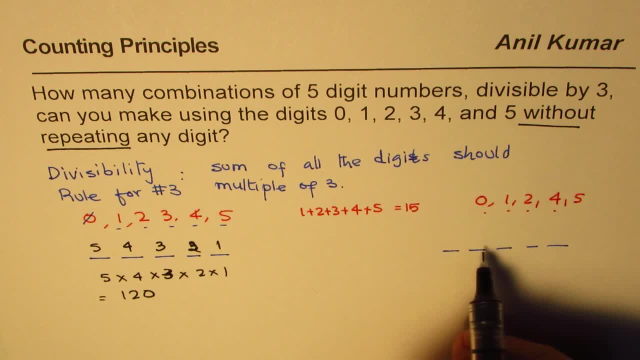 side I cannot place 0,. then we are left with 4 digit number, not a 5 digit number right. So here we cannot place 4, we have a choice to select a number from only these 4 of them. 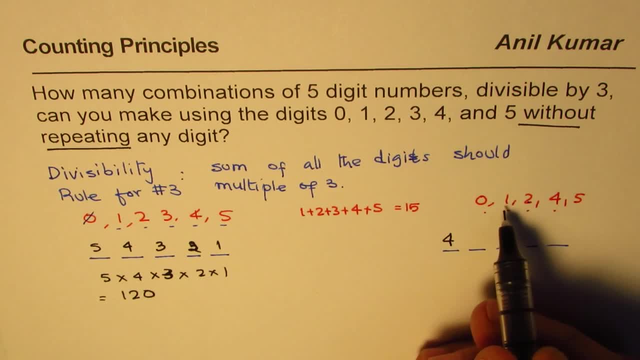 so it can be filled by one of these 4.. Once we place one of these 4 here, we are left with another 4 set of numbers, including 0, and once we place 0 or any other number, 2 numbers have been occupied, so we are left. 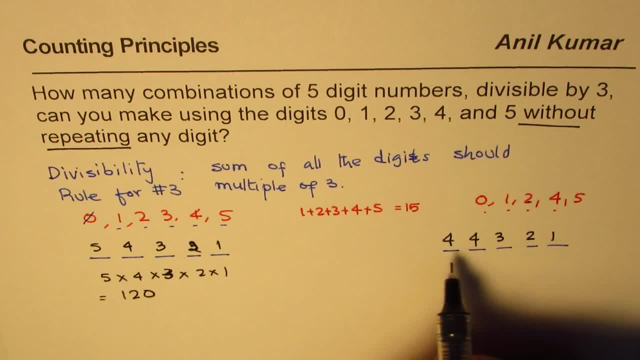 with 3.. Once 3 are occupied, 2 and 1, so that becomes the combination for us: 4 times 4 times 3 times 2 times 1, that is 4 times 4 is 16 times 3 is 48, and double of that is 96.. 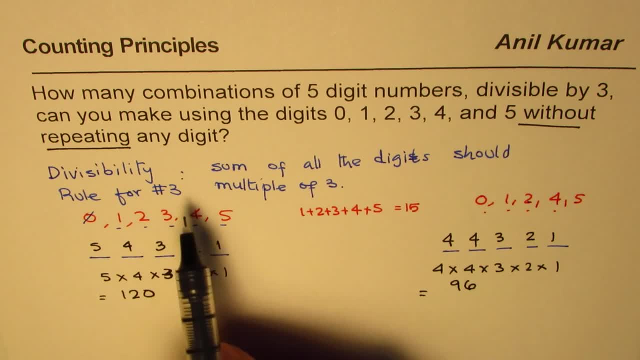 Now, can you make a 5 digit multiple of 3 by taking away 4 or 5?? The answer is no, Since if I take away 4 from 15, I am left with 11, and if I take away 5, I am left with. 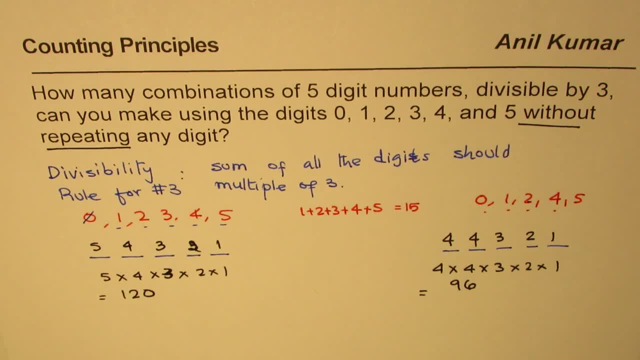 10 as sum of the digits, And 10 and 11 are not the multiples of 3, correct? So these are the two ways we can do it and those two ways. let's add them both. So what do we get? 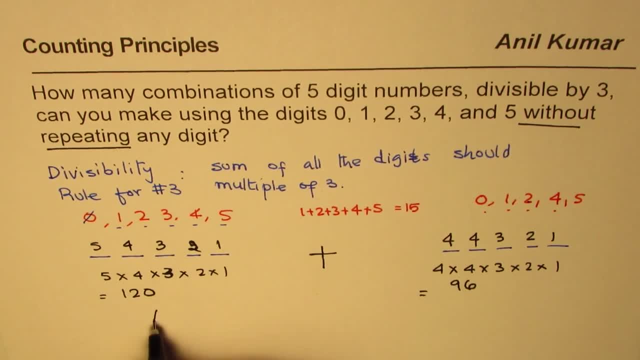 We get all the combinations of 5 digit numbers and that is our answer. So combinations are 120 and 1.. Plus 9 is 6,, correct, and when you add this you get what? 9 plus 2 is 11, and 2 here 216.